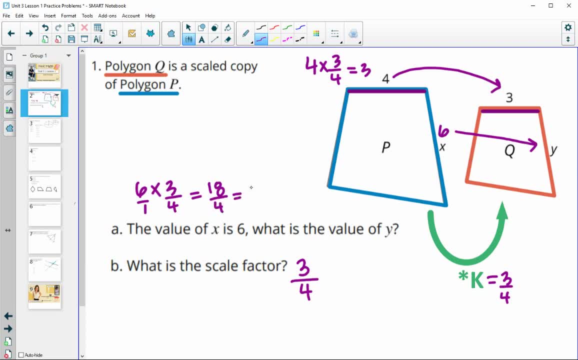 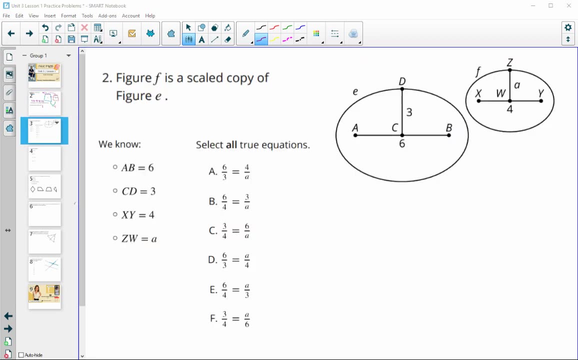 18 over 4, which is 9 over 2. if we wanted it simplified as a fraction or as a decimal would be 4.5.. All right, then in number two, we again have a scaled copy here, So F is the scaled copy. 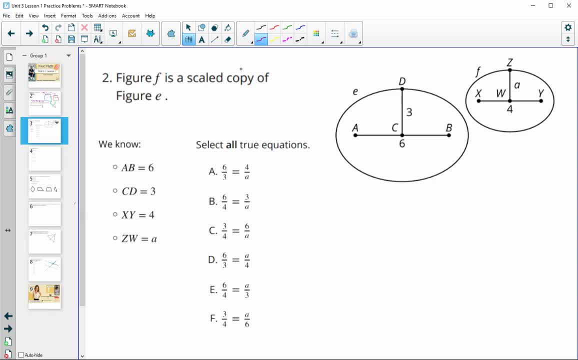 of E, And so we can see that that image is getting smaller than they told us. A bunch of different information that we know, And so we know that this segment here, AB, is 6. And we know that CD is 3. So I'm just going to make those purple in that shape And then in the scaled copy. 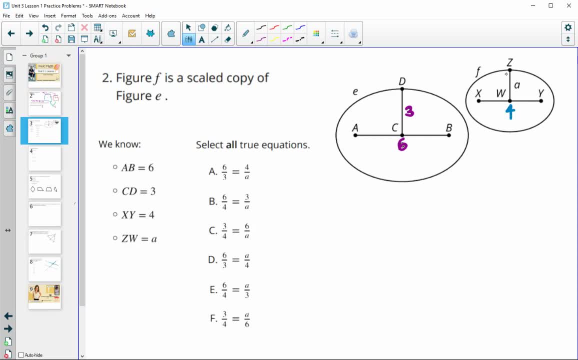 we know that XY is 4. And we also know that ZW is A, So they didn't give us an actual length for that, And so now it asks us to select all of the true values, And so we can see that we have a. 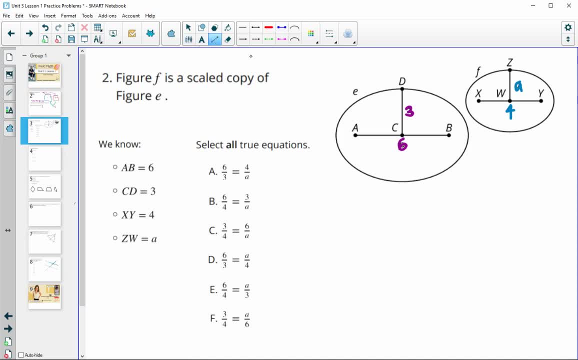 set of equations So you kind of just have to follow a pattern here. So let's take a look at what this first one does. So this first one had us look at 6 compared to 3.. So this kind of horizontal segment divided by this vertical segment, in this first shape. Then it said: 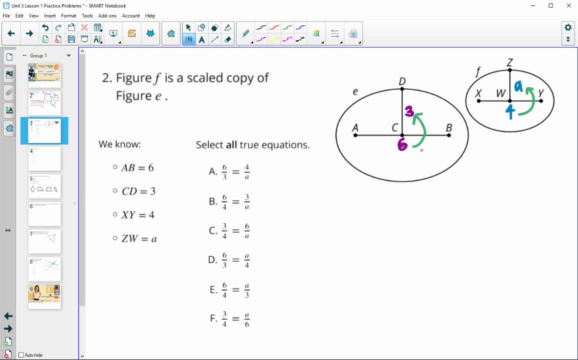 so 6 divided by 3 is the same as 4 divided by 8.. That's going to be true because we compared corresponding parts. So we went horizontal divided by vertical in the original And then horizontal divided by vertical in our scale. So that is going to create a true proportion. 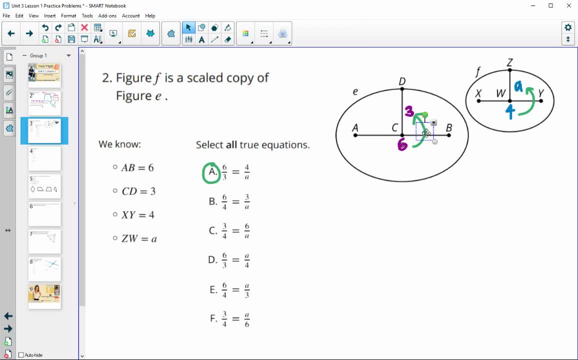 So then in this next one- and let me just get these out of here- The next proportion says 6 over 4.. So now we're comparing the horizontal in the original To the horizontal in the scaled. And then they said equals 3 over A. So you can see when I put. 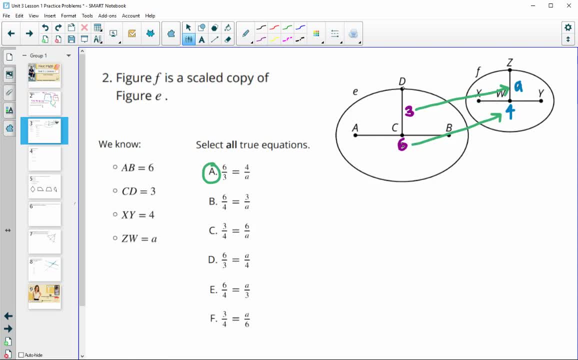 these arrows on, I'm saying comparing horizontal to horizontal And then vertical to vertical, And they're following a pattern. So this is going to be another true proportion, And once you have a true proportion you can kind of look at the cross products as well. So if we look at this, 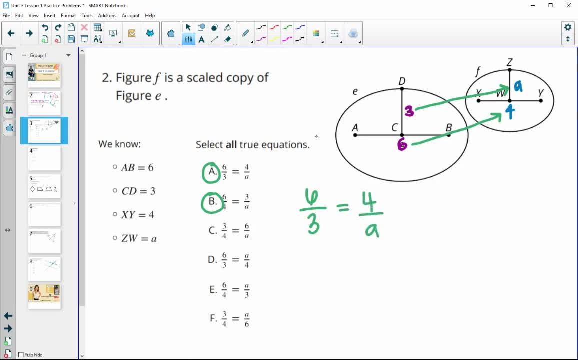 first one we say 6 over 3.. And we say 4 over A. So if these diagonals or these cross products end up being the same number, So 6 and A on that one And then 4 and 3 on this one, If we see that, we'll have a true proportion. So in B we see that 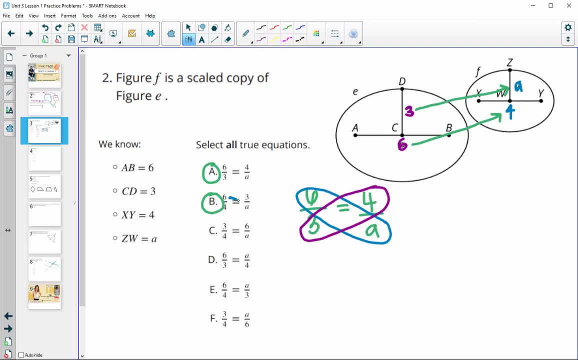 we still have 6 and A along this diagonal, And we still have 4 and 3 along that diagonal. So that's going to be good. So that's another strategy, All right, Then let's take a look at the rest. So for part C it says 3 over 4.. So now they're. 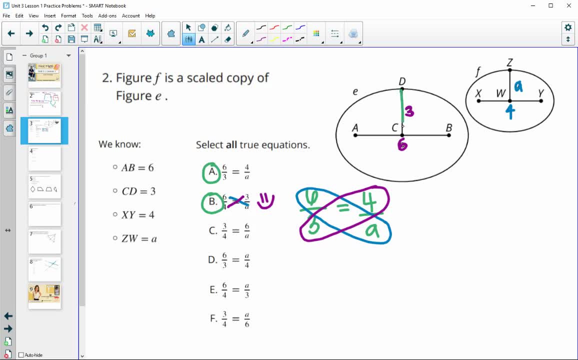 taking the vertical segment and comparing it to the horizontal in the other figure. So you can't do that where you're comparing a non-corresponding part in different figures. So this one just starts bad. And you could look at the cross products here again And you can see that the 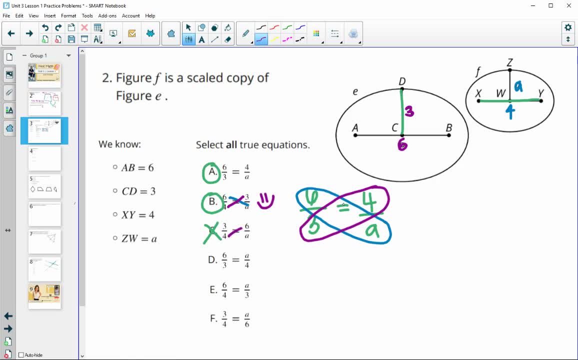 cross product has 4 and 6 on this, on the diagonal, Okay, And 4 and 6 don't go together. 6 goes with A, 4 goes with 3. So this one's going to be bad. D asks us to compare 6 to 3. And we can do that. 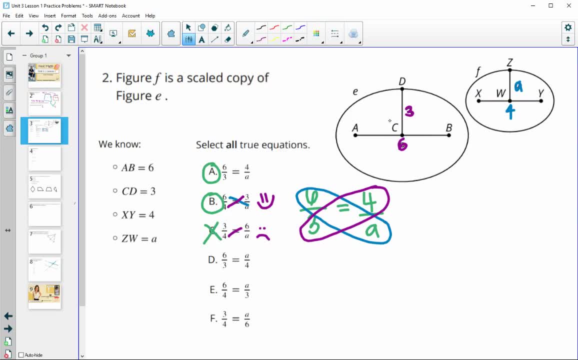 because it's within the same shape. So we're comparing horizontal to vertical. Then we just have to do the same thing in the other, So 6 to 3.. Now they did A and 6 to 3. So we're comparing. 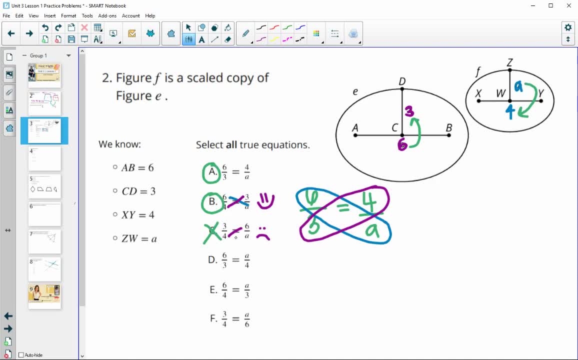 A to 4.. So now they flipped that around and went vertical to horizontal, So that one's going to be bad. We can again see that on the diagonal that they put that the wrong numbers are on the diagonal. E does 6 to 4, which is fine. We can compare horizontal in both shapes. So we're doing. 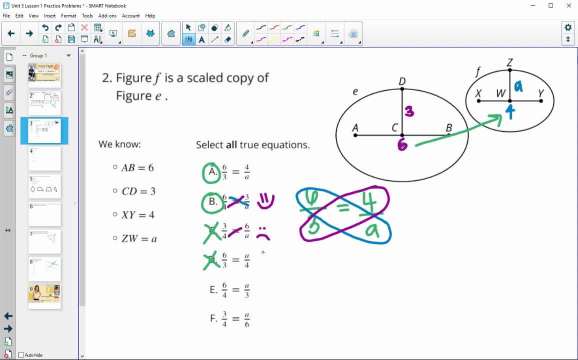 horizontal to horizontal, So 6 to 4.. Now they went A to 3. So we're comparing A to 3. So we're going to do A to 3.. They went backwards. Okay, So that's the wrong order. Final one: They did 3. 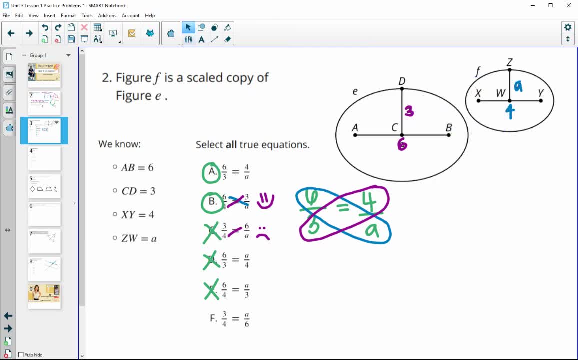 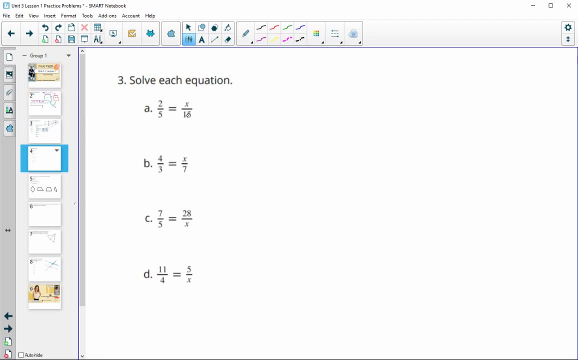 compared to 4. And that's comparing again the vertical in one to the horizontal in the other, So that one starts out bad. All right. Number 3 has us solving some proportions. So we're going to do cross products here, cross multiplication. 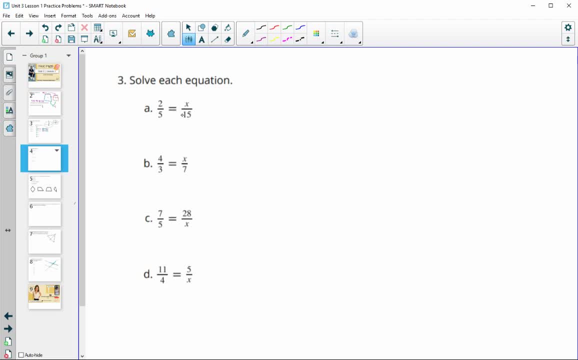 You can also do some other skills here, So I'll show you a couple different ways. So in this one you can do 2 times 15. So that's going to be 30. And I'm just going to write it out for you: 2 times 15.. And then, on this side, multiplying 5 times X. So then you would be. 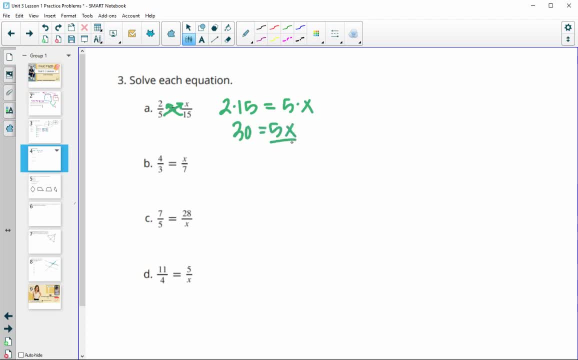 getting 30 equals 5X, And then you could divide by 5. And you would get 6 equals X for this first one. Another way you could have looked at that same problem. So we have 2 over 5 equals X over 15.. 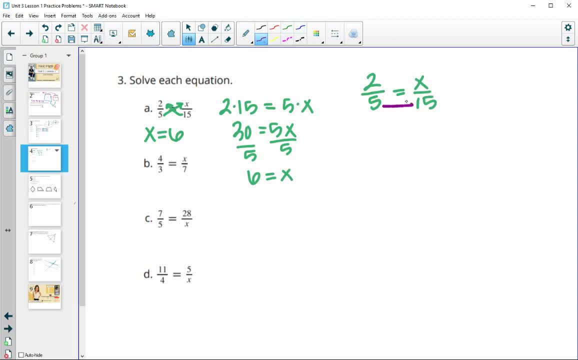 You could notice that on the bottom here, 5 times 3 gives us 15.. So we could apply the same idea to the top and multiply the top by 3. So 2 times 3 would give us the top over here of 6. So that's. 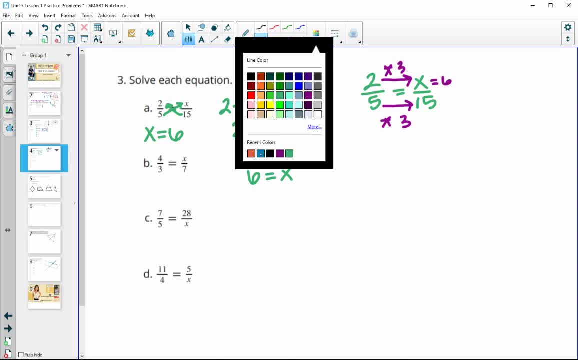 another way you could have looked at that one. All right, Then let's look at B. So I'm just going to write it over here. So we've got 4 over 3 equals X over 7.. Now, a nice number, does. 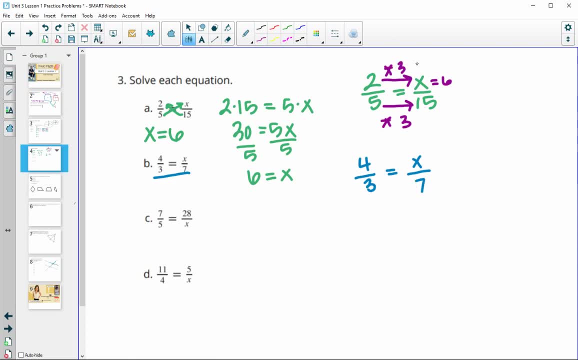 not take 3 times something to get 7.. So we probably can't really use this strategy as well. But we can cross multiply. So 7 times 4 is 28. And then we've got 3 times X, And then we can divide both sides. 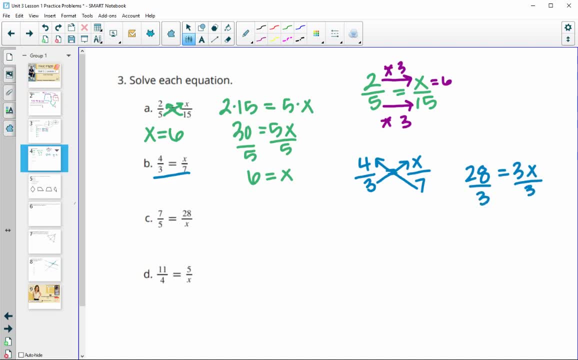 by 3.. When we do 28 divided by 3, we get that X equals 9.3 repeating, And so you can just put 9.3 or 9.3 with that little bar over it. All right, Then C. So again. now, this one does have some nice. 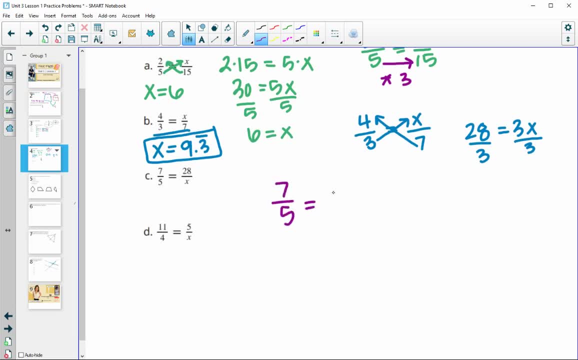 numbers up here with 7.. I'm just going to write it again: 7 over 5 equals 28 over X. So we can see on this top one here: 7 times 4 gives us 28.. So we could use that idea for the bottom and do 5. 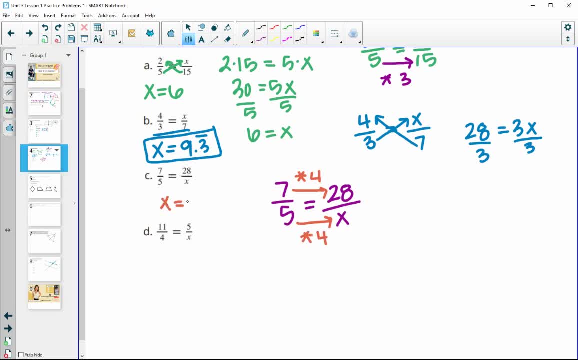 times 4. And then we would get X equals 20. So you could do that Or you could cross multiply. So if you cross multiply, you're getting X times 7. And then 5 times 28 is 140.. 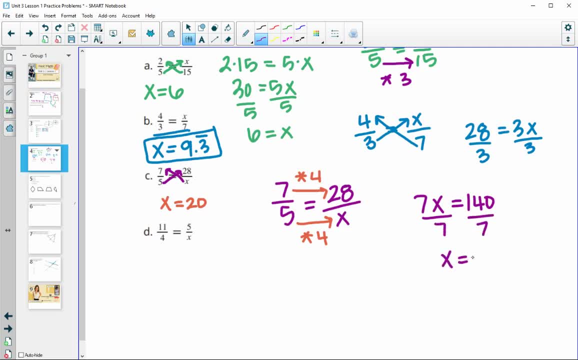 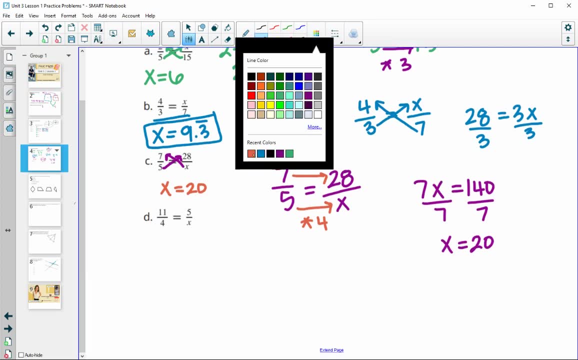 And then you could do that, So you could do that, So you could do that, So you could do that, And then you could divide by 7 and get X equals 20.. So either way is fine. And then final one here. 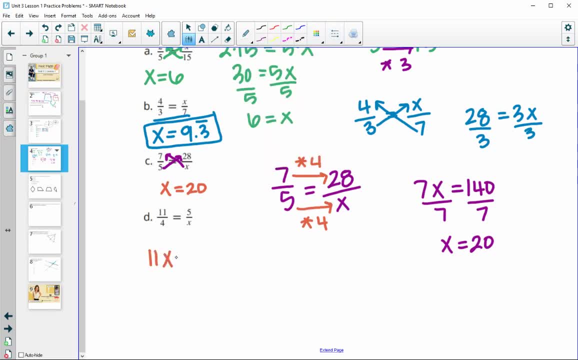 So we can do: X times 11 is 11X, And then 4 times 5 is 20.. Divide both sides by 11. And we would get X equals 1.818181. repeating. So, if you wanted to round that to the nearest hundredth, you'd get 1.82.. 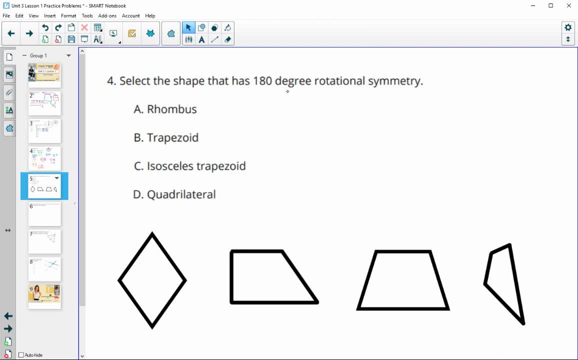 All right. Number four asks us select a shape that has 180 degree rotational symmetry. I've drawn the shapes down here to kind of help us visualize this. So this first one is a rhombus. So I'm just going to change the color here And I'm going to just try rotating these 180. So 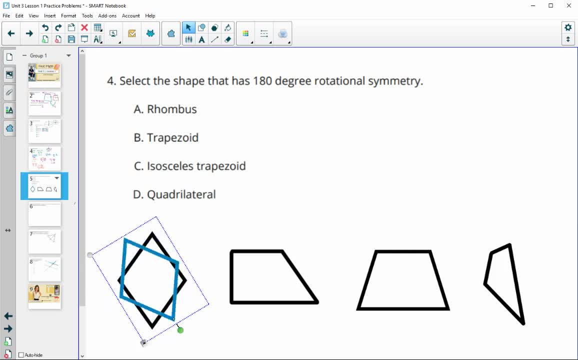 it's going to be moving my rhombus And then I'm going to try rotating these 180.. So I'm going to to be moving my green dot all the way down to the bottom. So I'm going to rotate 180 and we see that. 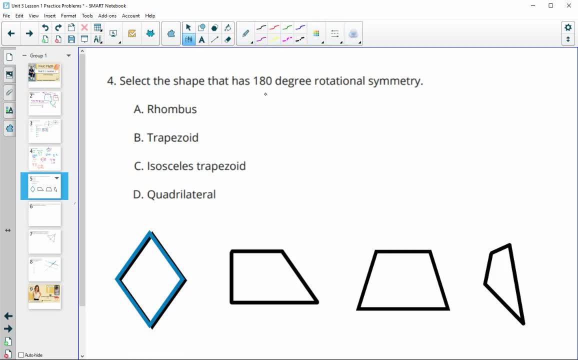 the rhombus lands on itself, So that one would be good That one does have rotational symmetry. and this said, just select the answer. So there's only one answer. So that's the answer. But I do want to show you on these other ones that they don't have 180 degree rotational. So B is just a. 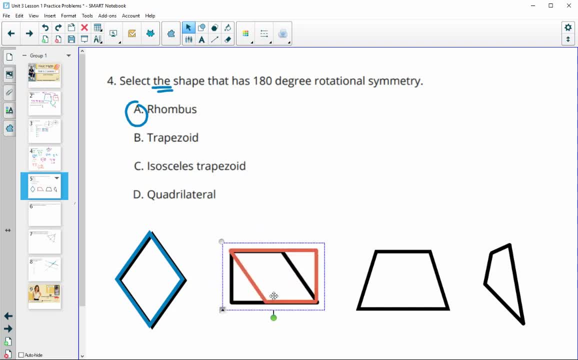 trapezoid, So I'm going to rotate this 180 and see that it does not land on itself. We'll do the same for this one. So now this one is an isosceles trapezoid, meaning that these two 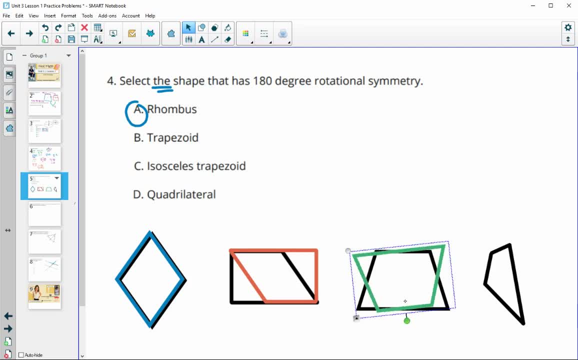 legs are the same size, So we'll rotate 180, see that that does not land on itself. And then the last one. they just wanted any random quadrilateral, So I just made one up. Could be anything but rotate 180 degrees. 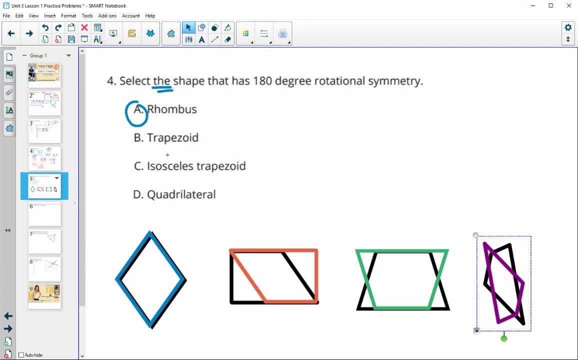 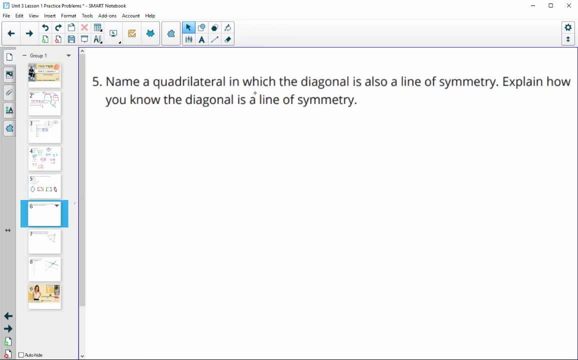 And we will see that again, that one did not land on itself. So the only one of these four options that does is the rhombus Number five. name a quadrilateral in which the diagonal is also a line of symmetry and explain how you know. So this one could be a square or a rhombus. 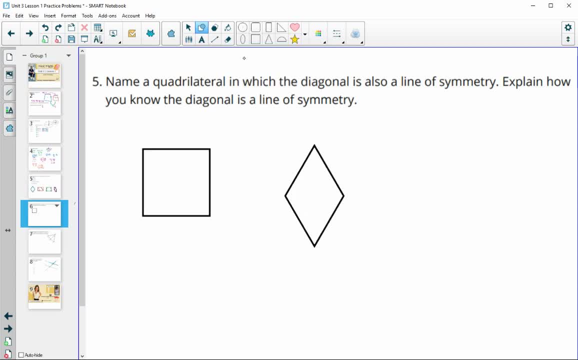 And let me get a rhombus on here. And we know that a square is actually also a rhombus, because the rhombus just has the equal sides, And so a square would work for this as well. So either of these two shapes is fine. Let me just draw in a line of symmetry or a diagonal, that's. 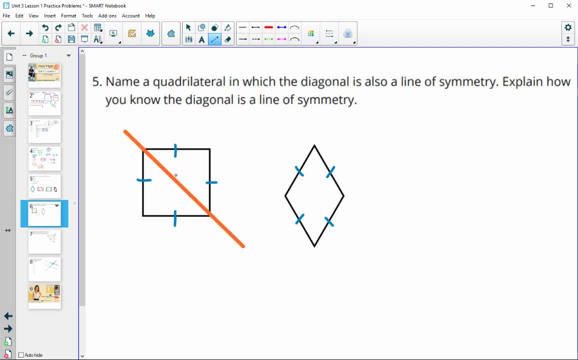 also a line of symmetry. So we know that these two triangles are exactly the same because the diagonal would be equal. So side, side, side would flip that kind of back on itself. And the same thing with the rhombus. So if we did this diagonal, 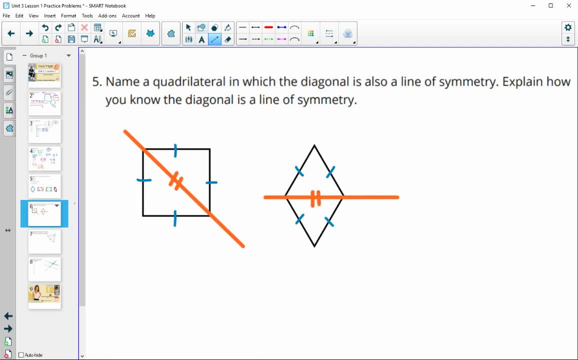 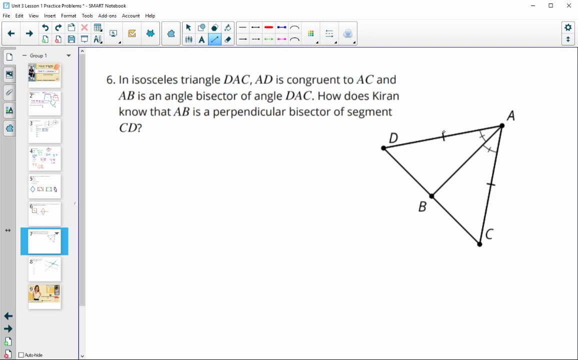 we see the top triangle is identical to the bottom triangle through side, side, side, And so then it's just going to flip over on itself or reflect over that line. Number six, we have an isosceles triangle shown here. They tell us a couple of things. 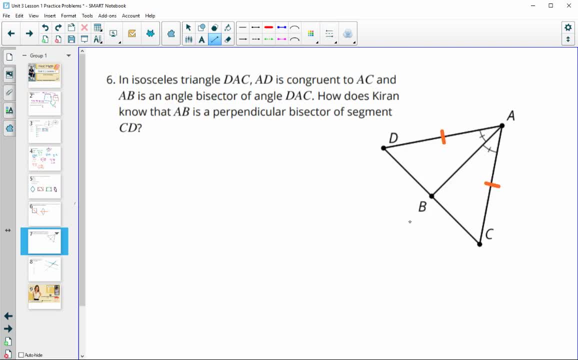 We know that this side is congruent to this side And we also know that this line in here is the angle bisector, So this angle is congruent to this side angle. So how does Kieran know that AB is the perpendicular bisector? So how do we know that? 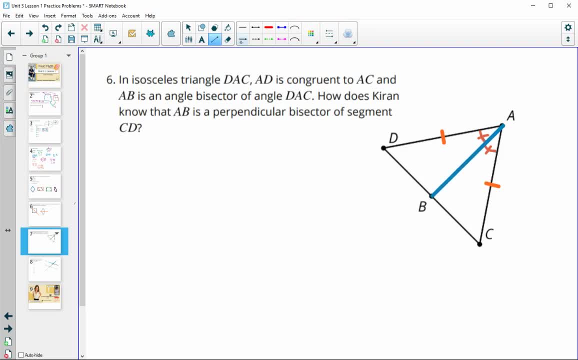 this is also the perpendicular bisector, not just the angle bisector, And so we can look at this: AB is in both of these two triangles, So we know that it's the same segment in each triangle, So it's the same, And then that shows us. so if I just kind of 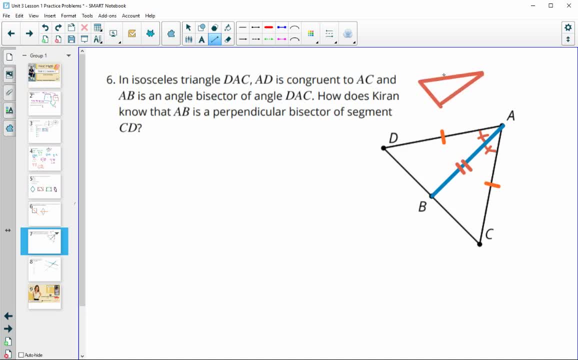 redraw this top triangle. we've got this stuff marked. We've got this and this equal in the other triangle as well as this angle. So we know that the two triangles are congruent by side angle side, which means that if those two triangles are congruent, now we know that. 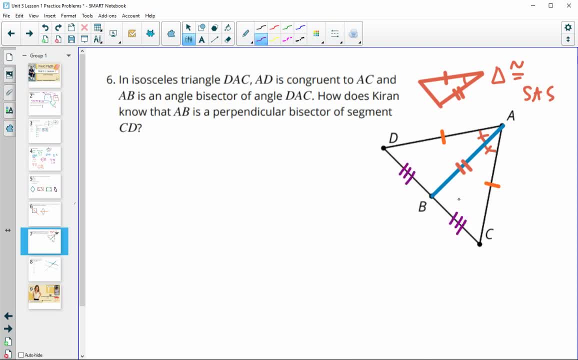 this piece is congruent to this piece because of the corresponding parts. So once we know the triangles are congruent, we know that the triangles are congruent, So we know that the triangles are congruent. So once we know the triangles are congruent, we know that the 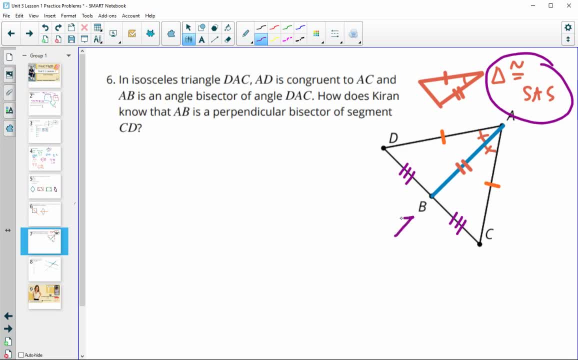 triangles are congruent. We know their parts are congruent. So that would mean that B is definitely the midpoint, So it is bisecting it. So that proves the bisector part. And then to get the fact that it's perpendicular, you've got a couple of options. So we know it's perpendicular. 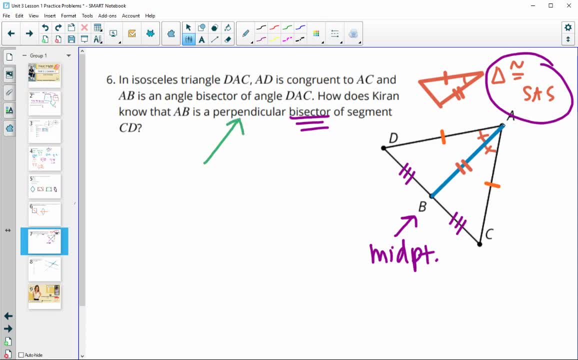 because A is equidistant from both C and D. So we know that A is on the perpendicular bisector. Okay, so we know that A is on the perpendicular bisector. So we know that A is on the perpendicular bisector. Okay, so we know that A is on the perpendicular bisector. Okay, so we know that. 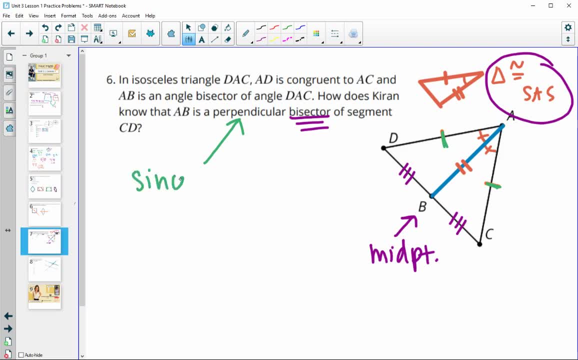 that blue line would be the perpendicular bisector, since A is equidistant from C and D. So that's one way you could say it. Another way you could look at this is: you know that this angle here and this angle here are equal to each other, since they're corresponding parts, And we know that a straight 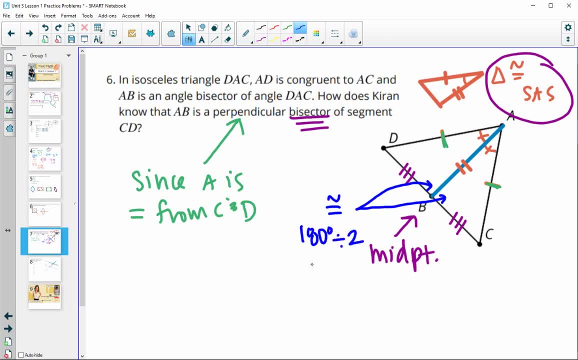 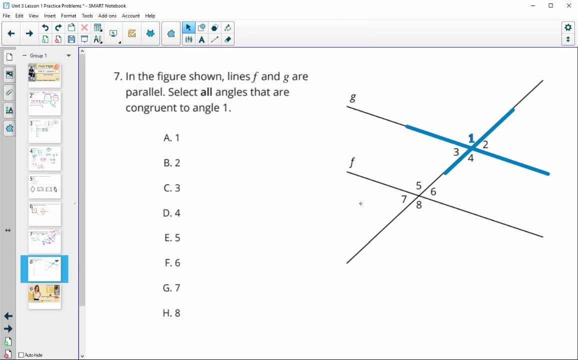 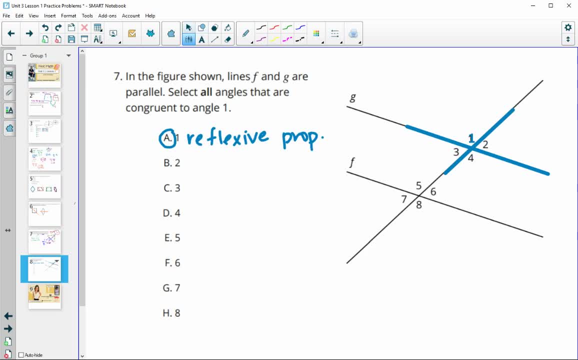 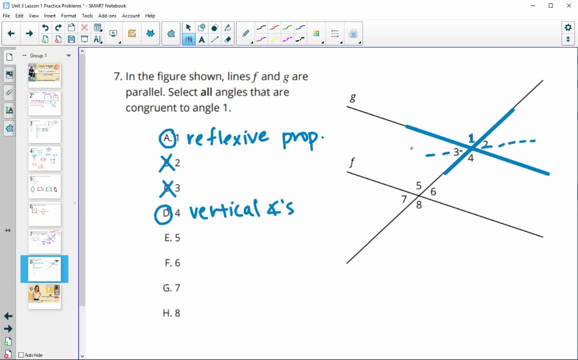 So if those two angles are equal, then we know that A is on the perpendicular bis. So if those two angles are equal, then we know that A is on the perpendicular bis would have to equal 180. And same with 7.. Okay, so not equal to angle 7.. So we would know again: angle 1 is equal to angle 5 by corresponding, and then 5 and 7 are next to each other, So 1 and 7 would be 180 instead of equal to each other. 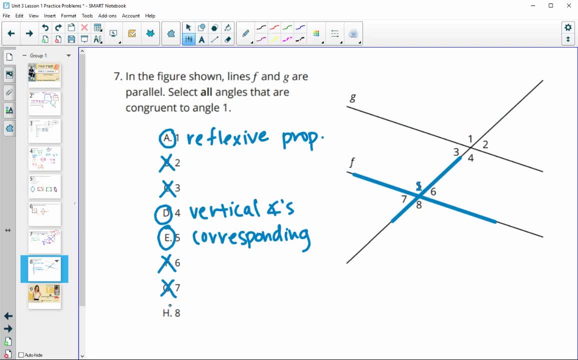 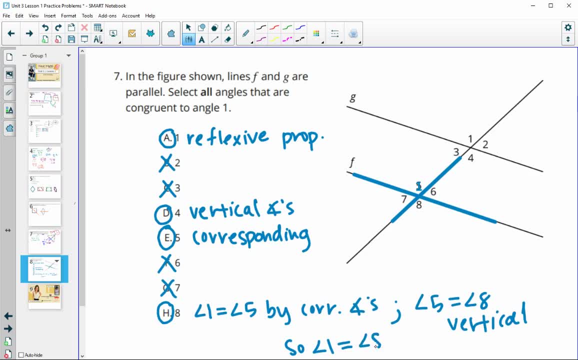 So angle 1 would have to equal angle 8..